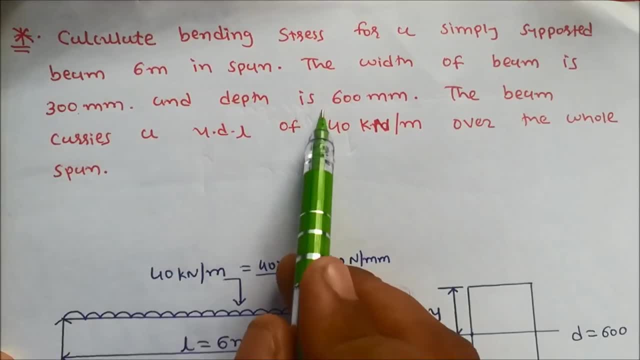 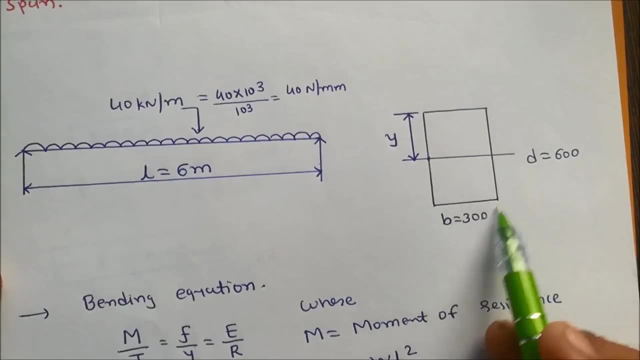 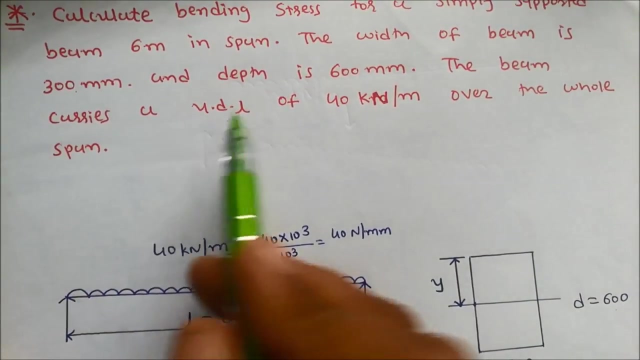 beam is 300 mm and depth is 600 mm. So width is given, b is equal to 300 mm and depth is given b is equal to 600 mm. Then data is given. the beam carried a UDL of 40 kilo Newton per. 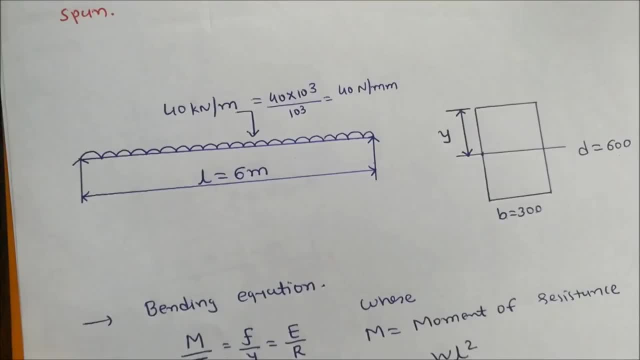 meter over the entire span Means here UDL over entire span. that is given 40 kilo Newton per meter. So here 40 kilo Newton per meter. So convert it into Newton. So 40 multiplied 10 raise to 3, and per meter instead of meter we convert it into mm. So divided by 10 raise to 3.. 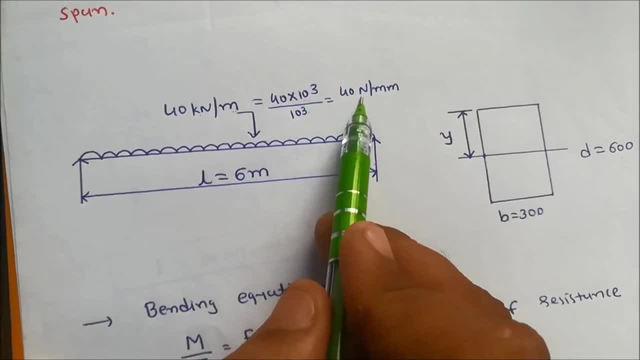 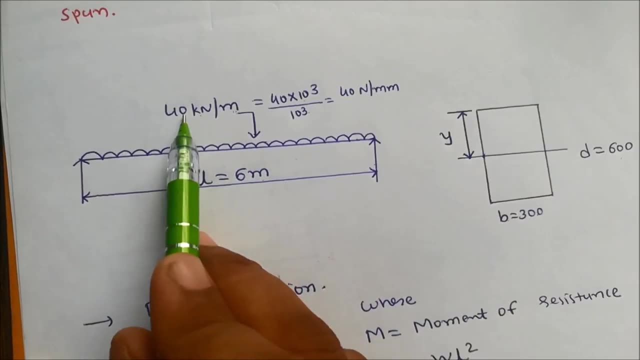 So 10 raise to 3,, 10 raise to 3, cancel out. So 40 Newton per mm. So here simply supported beam is given, length is 6 meter, UDL is given, that is 40 Newton per mm. Section is given. 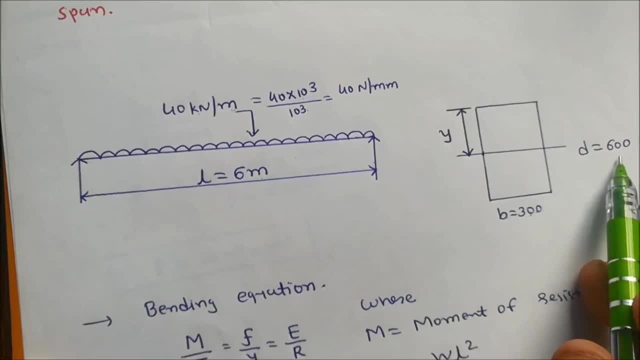 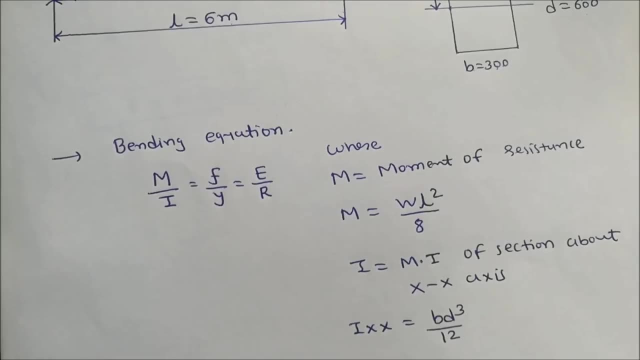 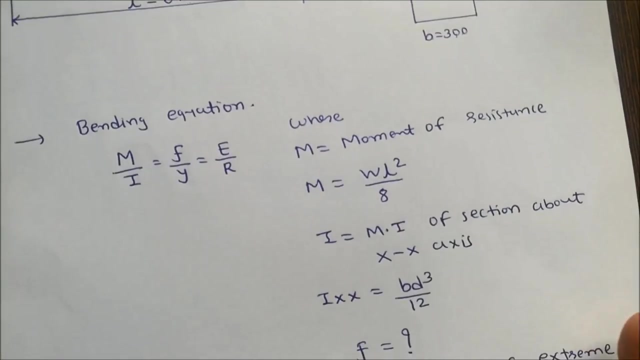 width is 300 mm And we find bending stress. We know bending equation that is M by I is equal to F by Y, is equal to E by R, Where M is equal to moment of resistance And for simply supported beam with UDL over entire span. we know that maximum bending moment, that is M, is equal to W L square. 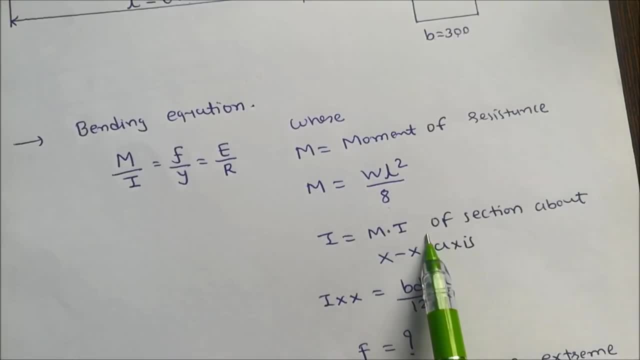 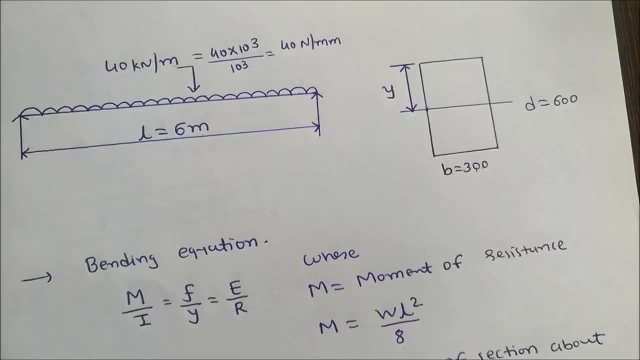 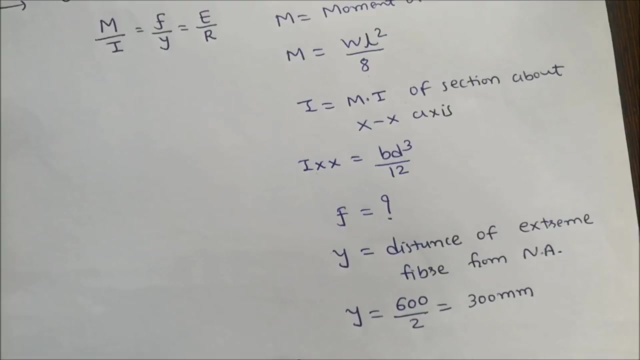 by 8. Here I means moment of inertia of section about x-axis, So I x-axis. we know that moment of inertia for rectangular section, that is BD cube by 12. So I x-axis is equal to BD cube by 12.. Here we have to calculate. bending stress means. 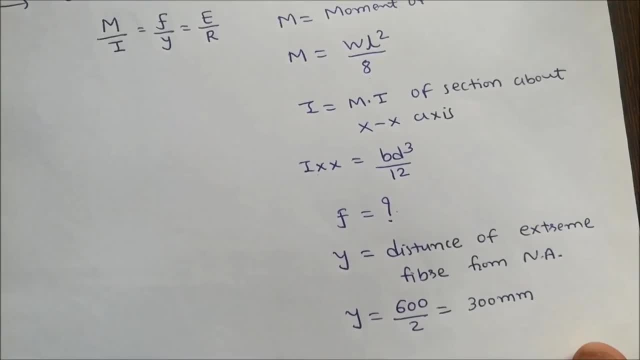 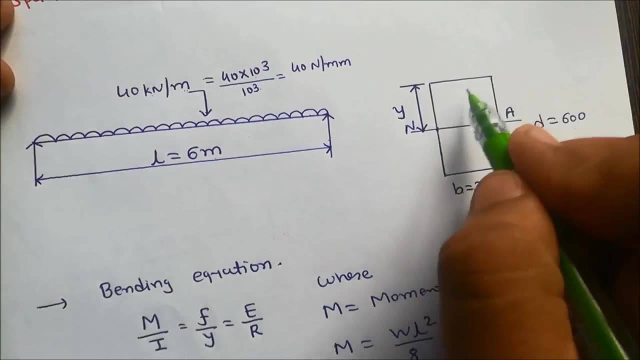 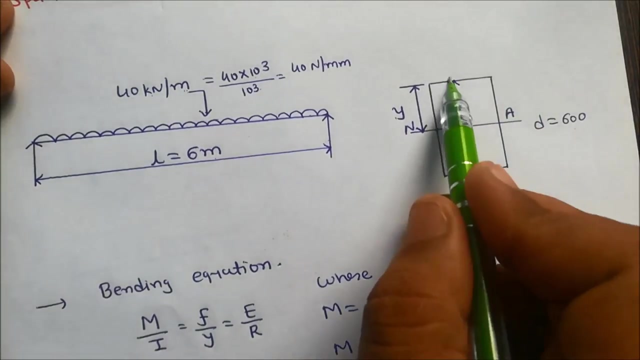 F we calculate and Y means distance of extreme fiber from the neutral axis. So here it is neutral axis and distance of this is known as a Y, So distance of extreme fiber from neutral axis. So total depth is given 600 mm. So Y is equal to 600 divided by 2. that 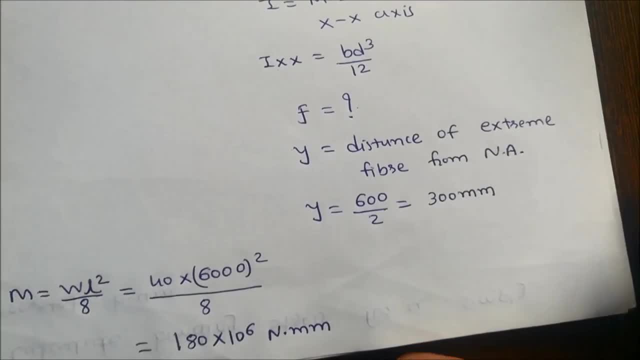 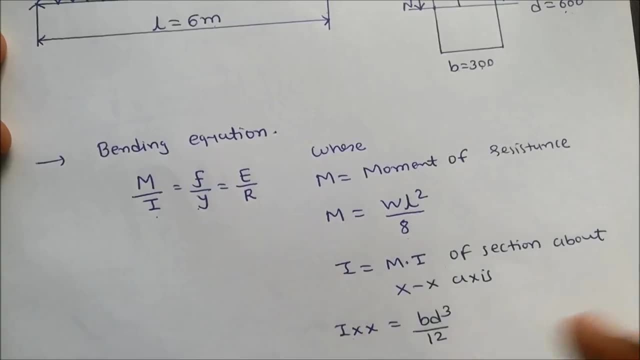 is 300 mm. So Y is equal to 600 by 2, that is 300 mm. So here we simply put value of M, I and Y. So we know that M is equal to W L square by 8, because here simply supported.